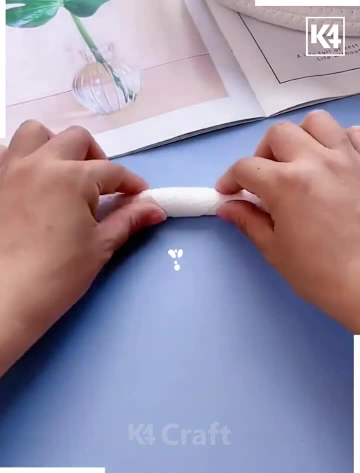 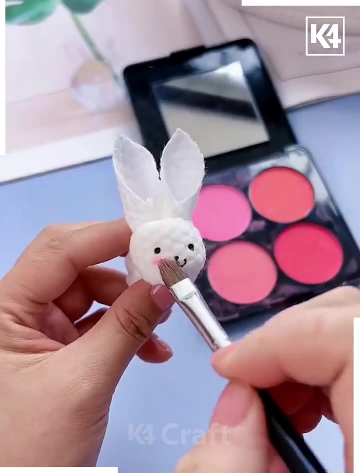 This next one, you're going to be making bunnies straight out of tissue paper and a little bit of eyeshadow. Can you believe that All you need is tissue paper, a rubber band, maybe a marker and eyeshadow? and how wonderfully that had turned out. 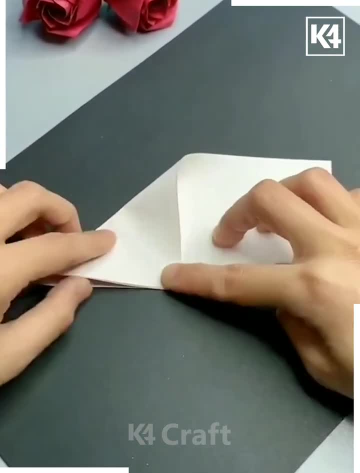 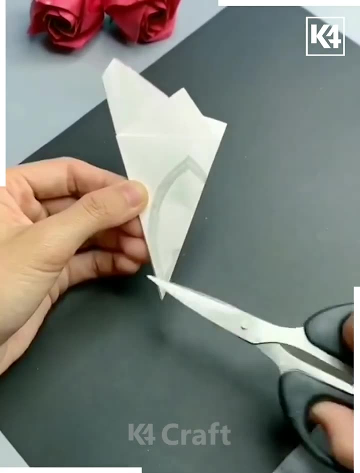 This next one is really quite easy to make, but it is a little complicated in terms of using scissors. If you're not familiar with using scissors, please do not attempt this. Be careful while using scissors. This can be used for stencils for other arts and crafts projects, and it's just so adorable to make. 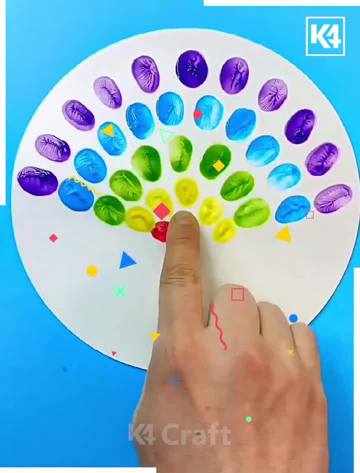 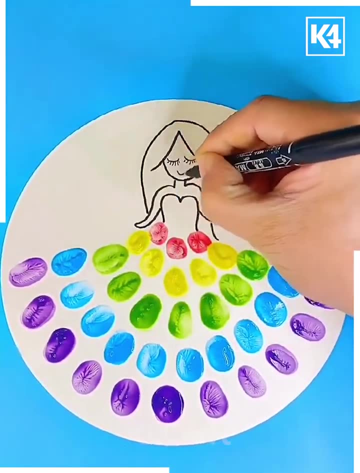 Now, this next one is really quite easy, and if you're looking for an easy way to make a little princess's dress, all you have to do is take some paint and use it as finger paint, Because it honestly gives it such a gorgeous effect. For this next one, you're going to be making semi-3d flowers, and for that you honestly just need sheets. 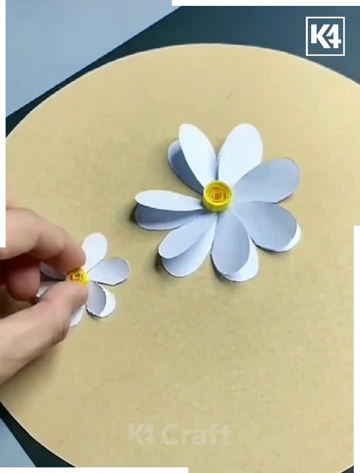 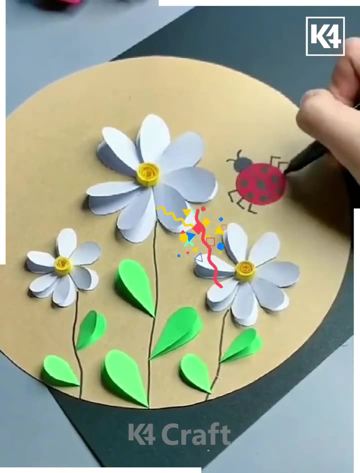 of paper and a little tactics on how you fold it. Look at how wonderfully that all tacks on. It's not even hard to make, it doesn't even take a lot of time, and once you've mastered it, you won't even need to look at this video. It's such a pretty set of flowers, don't you think? Comment down below. 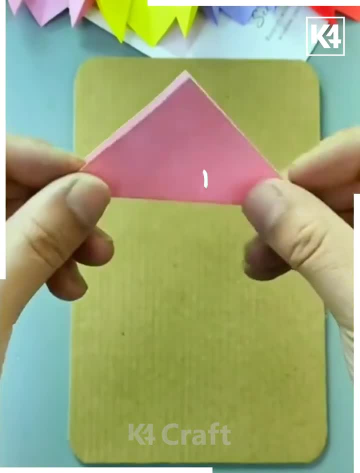 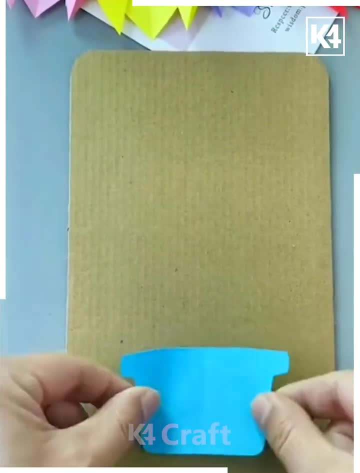 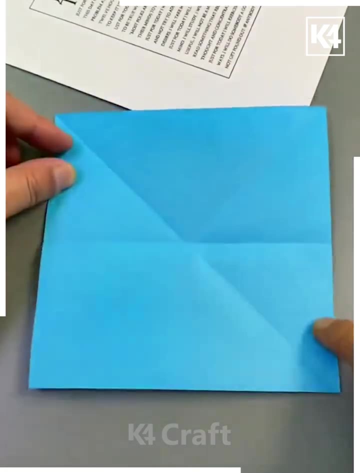 You need to fold it exactly like how the video shows you, and you can go ahead and use any color that you want for it. It's not even hard to make, it doesn't even take a lot of time, and once you've mastered it, you won't even need to look at this video in order to make it. And the surprising. 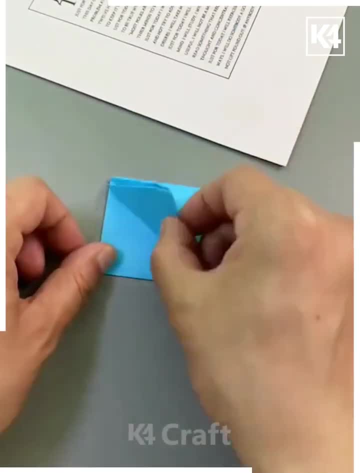 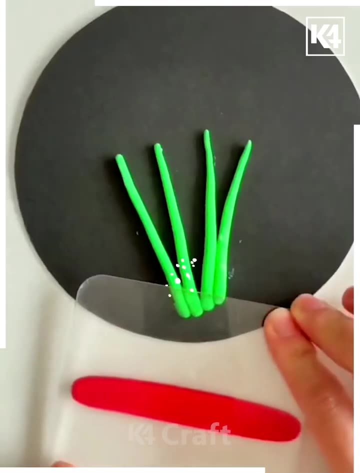 thing about this is that you can actually play with this sheet of paper that is folded. You can go ahead and spin it on the ground and look at how entertainingly it falls. This next one: you're going to be making a semi-3d set of bouquet flowers, So for this you're just 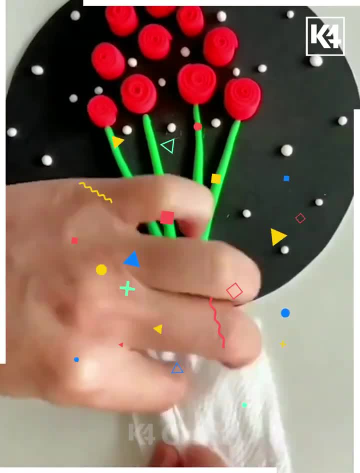 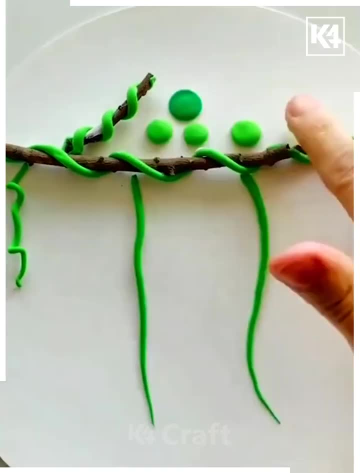 going to need a bunch of clay and a sheet of paper to make the bouquet. Doesn't that look amazing? For this next one, you're going to be making a semi-3d model out of clay for flowers. Doesn't that look amazing? All you really need is a bunch of clay in a different color, Doesn't that? 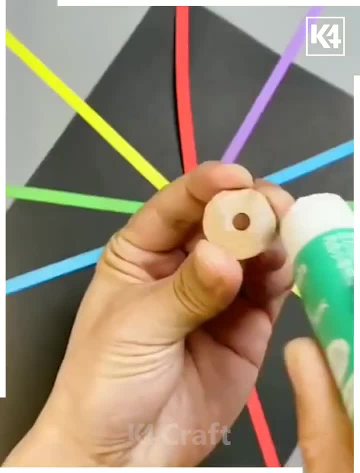 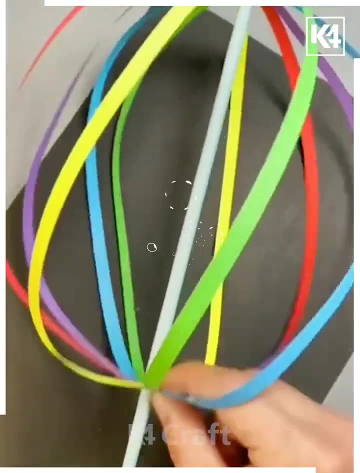 look amazing. Comment down below. Now, this next one is really just a colorful way to entertain yourself, and all you need is colorful strips of paper. All you have to do next is follow the instructions in this video and look at how cutely it turns out, Moving on to something that